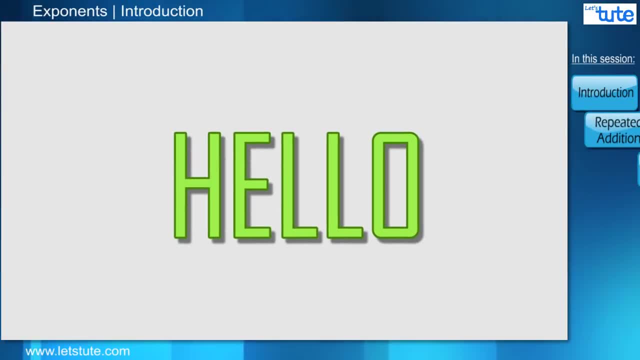 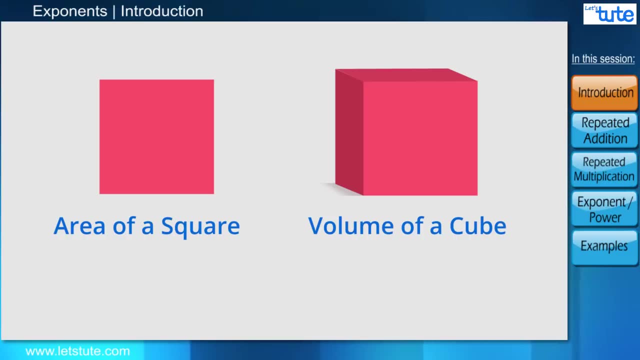 Hello everyone. do you know the area of a square or volume of a cube? Yes, you got it right. The area of a square is side square and volume of a cube is side cube. If the length of one side is A, then what will be the area of a square? Yes, it will be A square, Or suppose if we have a cube? 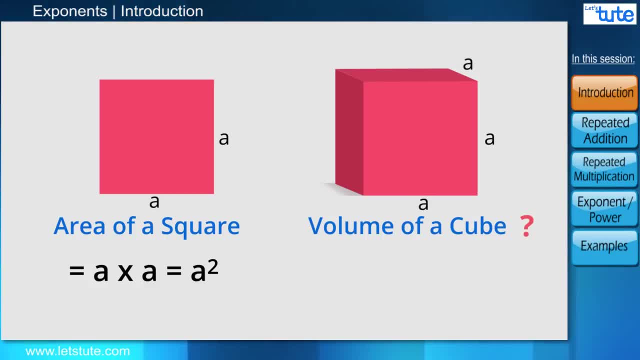 of length, A, then what will be the volume of a cube? Yes, it will be A cube, Friends. if you will see carefully, there is a number which is at the upper right corner of A. What does that mean? Hmm, we often came across this kind of numbers, but have you ever thought what exactly it indicates? 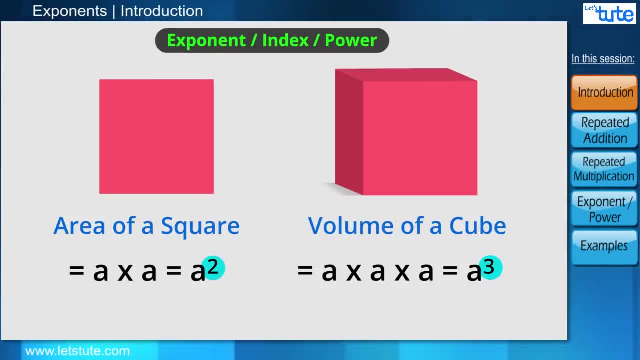 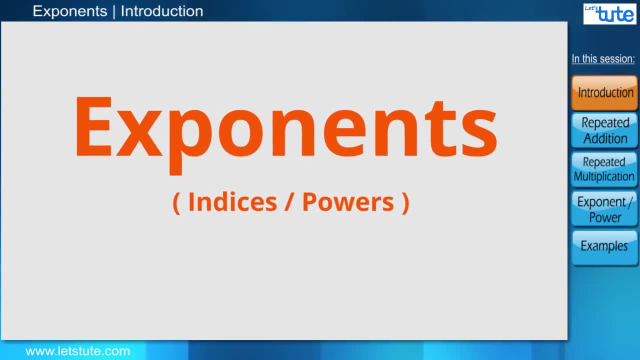 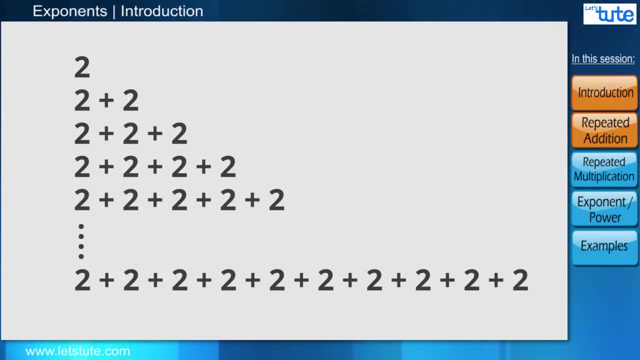 Well, friends, these numbers are nothing but the exponents, or index, or we can say power. So, friends, today in this session, we are going to explore more about the exponents. Okay, friends, let's have a look at these numbers. In first there is a single digit, 2,, next, 2 plus 2,, next 2 plus 2 plus 2, and so on. So, friends, 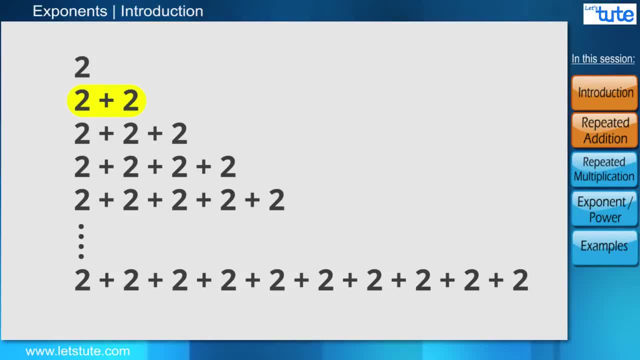 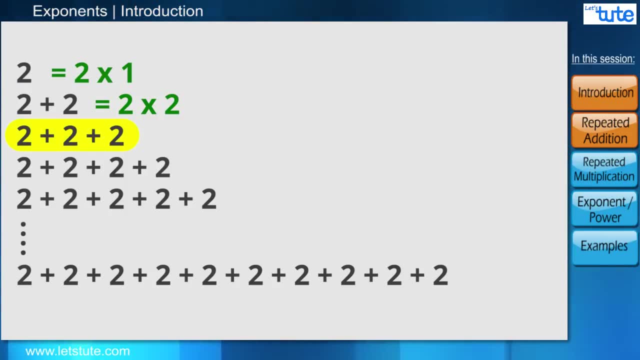 for this what we can do. If we have 2 plus 2, then we multiply 2 by 2, that is 2 into 2.. Similarly 2, then we can write it as 2 into 3 and so on. at the end you can see here, if we add 2 for 10 times. 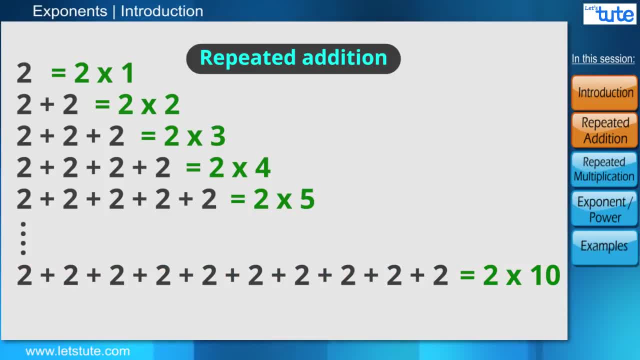 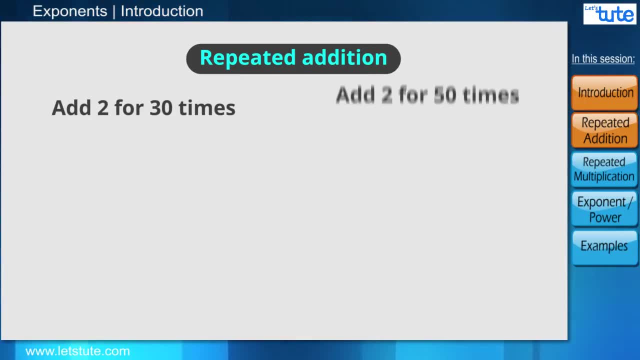 then we can write it as 2 into 10. this is known as repeated addition. now, if it is asked to add 2 for 30 times or 2 for 50 times, then how you are going to write it: 2 into 30 and 2 into 50. 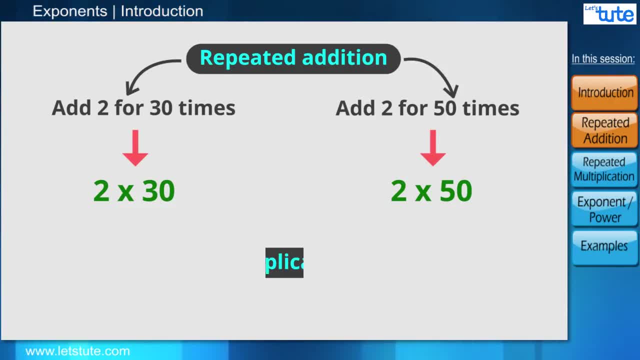 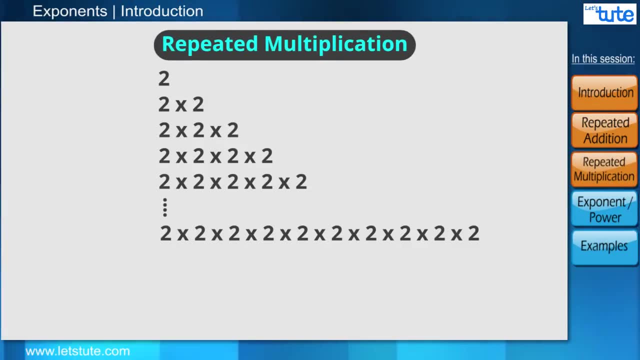 right, that means for repeated addition we can use multiplication. but what happens when we have repeated multiplication? let's have a look at these numbers well, at the end you can see 2 is multiplied 10 times. what if it is asked to multiply 2 for 50 times? are you going to write 2 for 50? 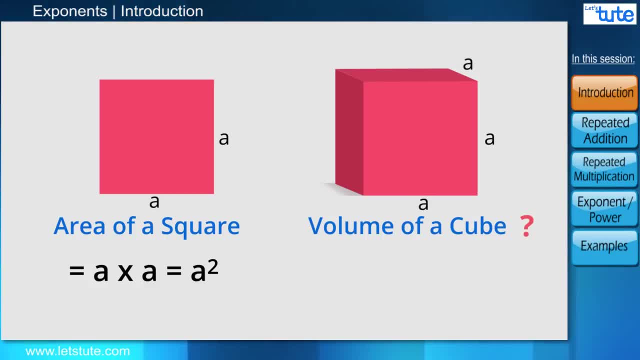 of length, A, then what will be the volume of a cube? Yes, it will be A cube, Friends. if you will see carefully, there is a number which is at the upper right corner of A. What does that mean? Hmm, we often came across this kind of numbers, but have you ever thought what exactly it indicates? 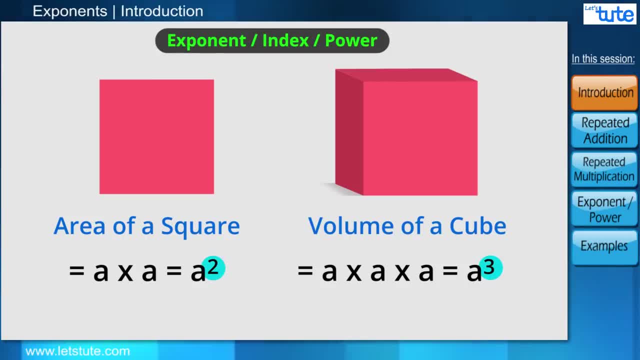 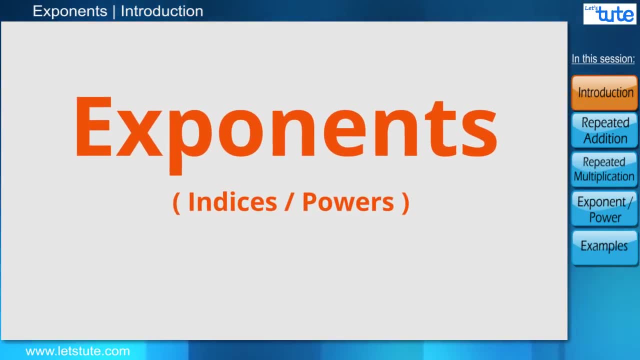 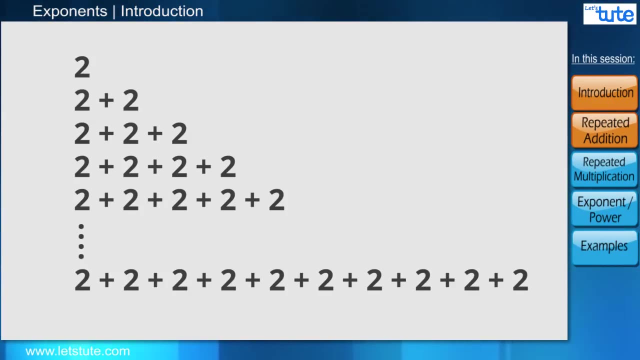 Well, friends, these numbers are nothing but the exponents, or index, or we can say, power. So, friends, today in this session, we are going to explore more about the exponents. Ok, friends, let's have a look at these numbers. In first there is a single digit, 2,. next, 2 plus 2,. 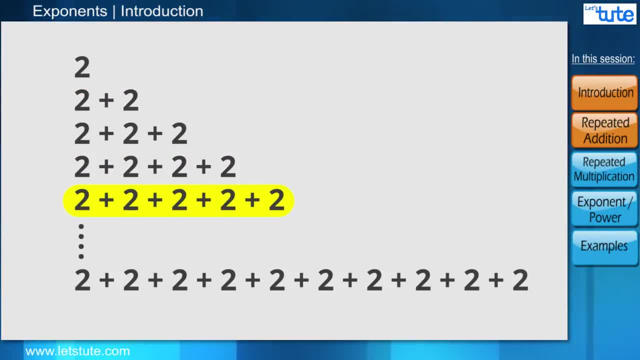 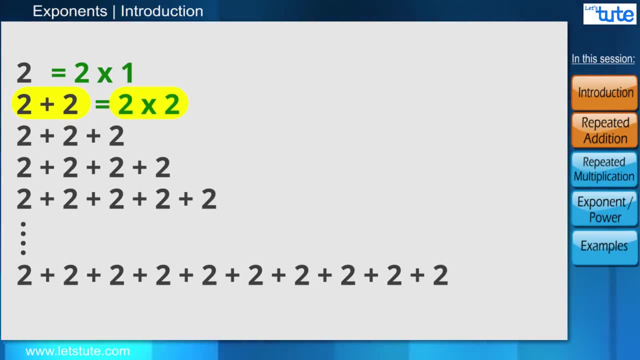 next 2 plus 2 plus 2, and so on. So, friends, for this what we can do, If we have 2 plus 2, then we multiply 2 by 2, that is 2 into 2.. Similarly, if it is 2 plus 2 plus 2,, 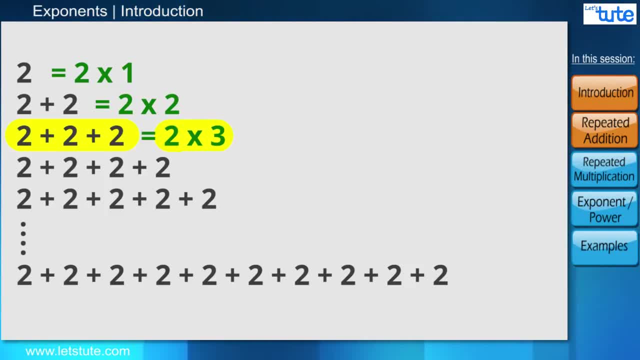 2, then we can write it as 2 into 3 and so on at the end. you can see here, if we add 2 for 10 times, then we can write it as 2 into 10. this is known as repeated addition. now, if it is asked to add, 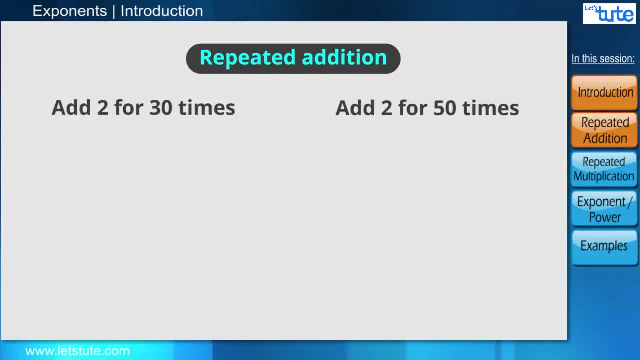 2 for 30 times or 2 for 50 times? then how you are going to write it: 2 into 30 and 2 into 50, right? that means for repeated addition, we can use multiplication. but what happens when we have repeated multiplication? let's have a look at these numbers. well, at the end you can see, 2 is 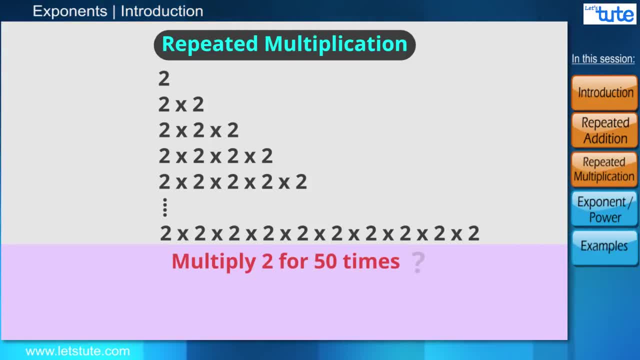 multiplied 10 times. what if it is asked to multiply 2 for 50 times? are you going to write 2 for 50 times? well, it is very time consuming and tedious process and it will be very difficult for counting and understanding. therefore, to avoid this lengthy operation, mathematicians have introduced this method. 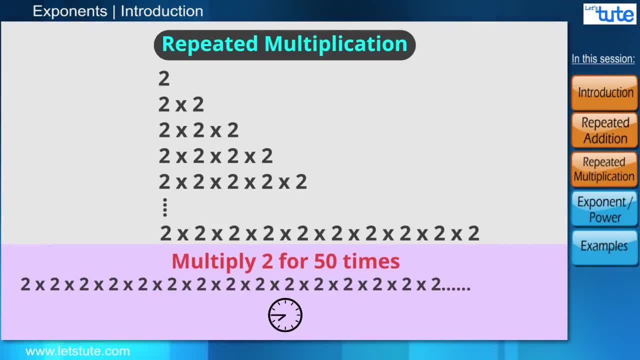 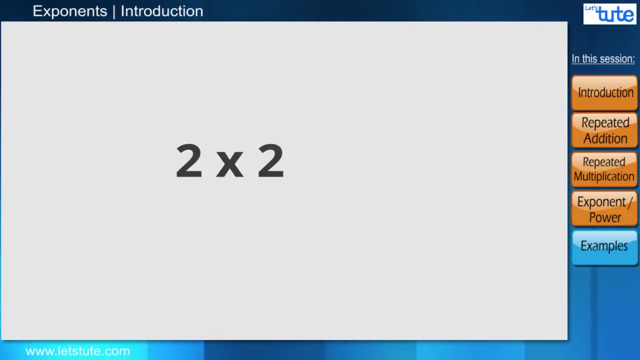 times. well, it is very time consuming and tedious process and it will be very difficult for counting and understanding. therefore, to avoid this lengthy operation, mathematicians have introduced this method. you can see here: if 2 is multiplied for 2 times, then it is written in the form of: 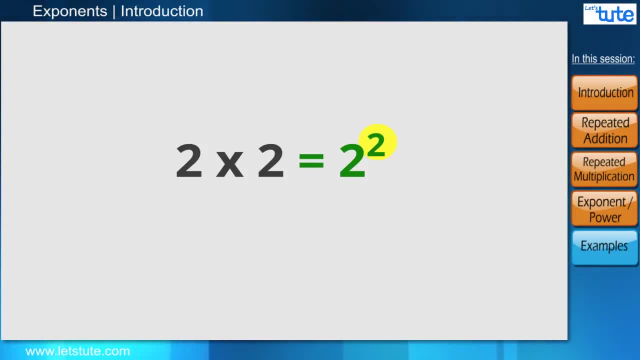 this mathematical operation, or you can say form, is known as exponent or power. the exponent is placed to the upper right corner of the base number and signifies how many times the base term is multiplied by itself. for example, you can see here: if 2 is multiplied for 2 times, then it is written in the form of: 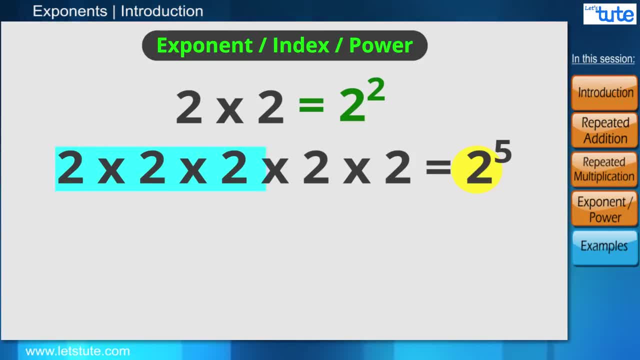 here you can see, 2 is multiplied for 5 times and 5 is exponent, as it signifies the number of times the number 2 has multiplied by itself. or you can say 2 to the power of 5 or 2 to the 5th power. 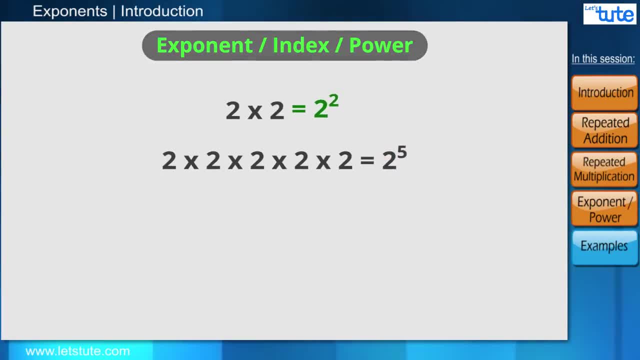 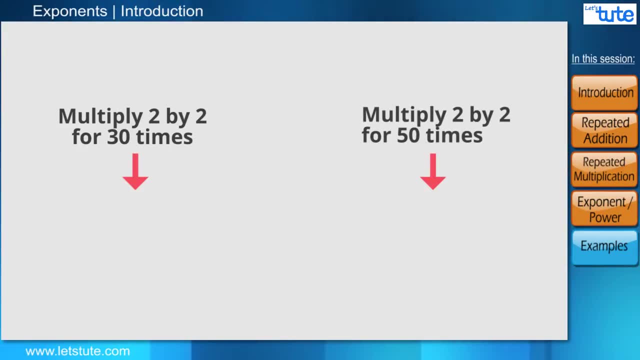 similarly, if it is asked to multiply 2 by 2 for 30 times or 2 by 2 for 50 times, then how you are going to write it: 2 raised to the power 30 and 2 raised to the power of 30 times, then it is written. 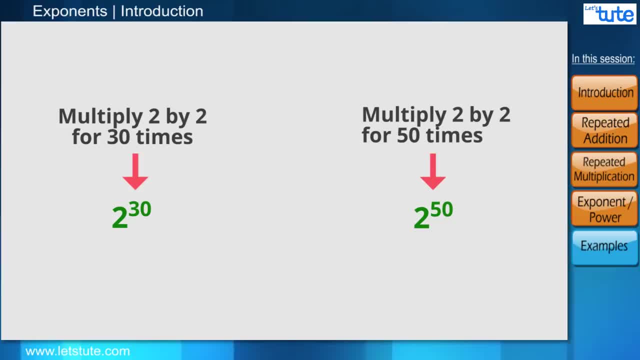 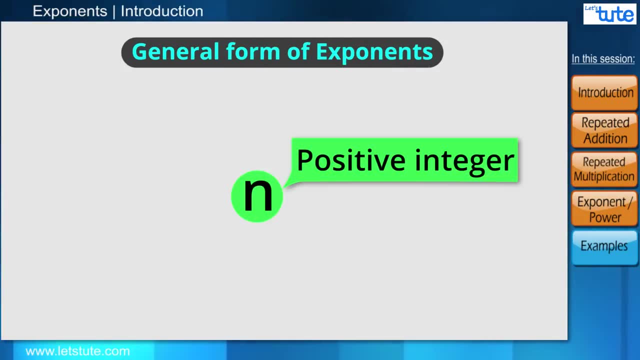 as 2 raised to the power of 50. right that means for repeated multiplication. we can use exponents in general form. if n is a positive integer and a is a real number, then a raised to the power of n corresponds to repeated multiplication. friends, there is also one more interesting. 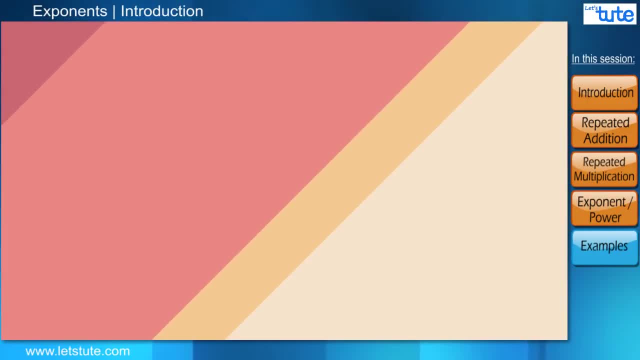 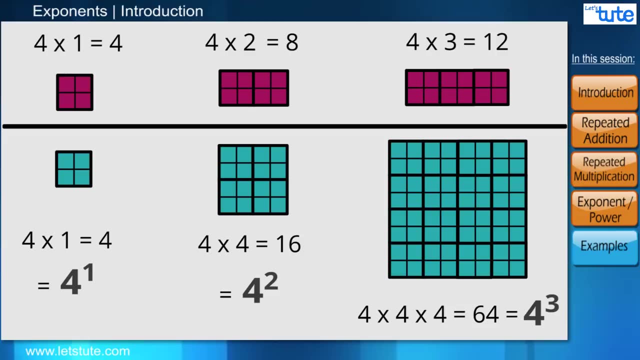 thing about multiplication and exponential. let's see what is that thing. let's have a look at this image. well, you can see here the number of boxes is increasing rapidly in exponential as compared to multiplication. here. exponentially means if something is increasing or expanding at a steady and usually rapid rate, then it is expressed using the exponents. we can even observe in our daily. 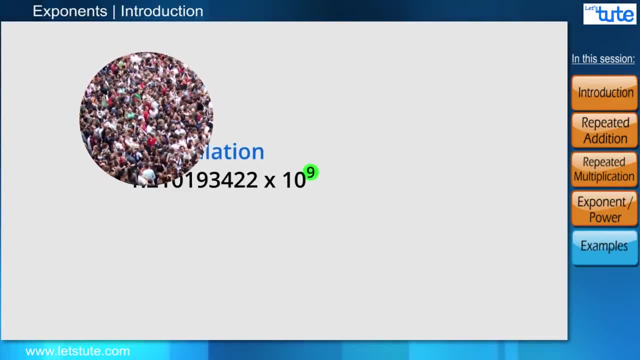 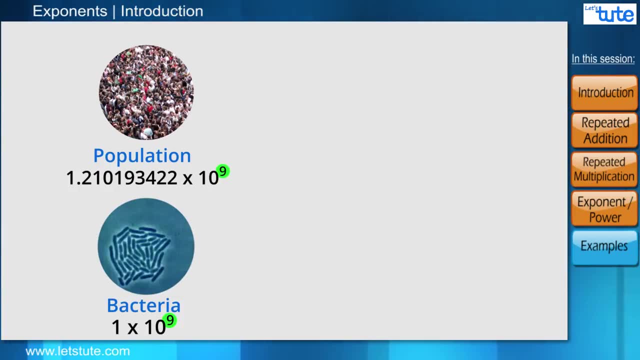 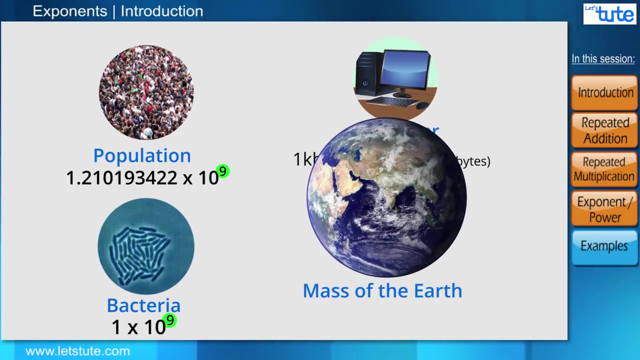 lives, like population grow exponentially each day, or growth of bacteria increases exponentially per hour. similarly, exponents are often used to describe how much memory or ram a computer holds. for example, 1 Kb equal to 2, raised to the power 10 bytes or 1024 bytes, or mass of the Earth is almost. 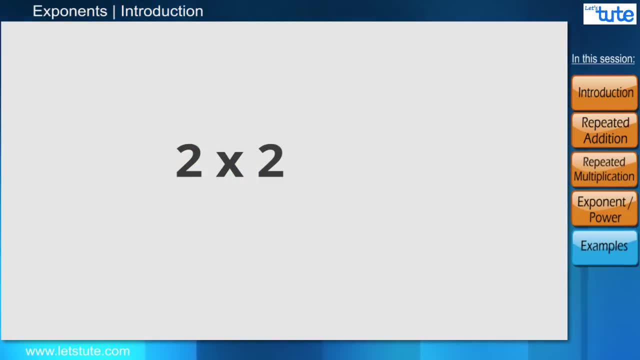 you can see here, if 2 is multiplied for 2 times, then it is written in the form of this mathematical operation, or you can say form is known as exponent or power. the exponent is placed to the upper right corner of the base number and signifies how many times the base. 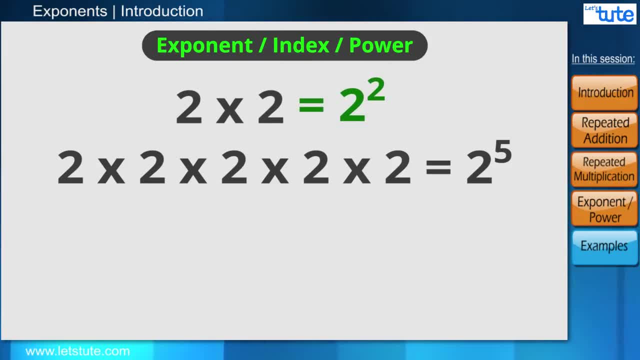 term is multiplied by itself. for example, you can see here: if 2 is multiplied for 2 times, then it is written in the form of this mathematical: here you can see: 2 is multiplied for 5 times and 5 is exponent, as it signifies the number of times. 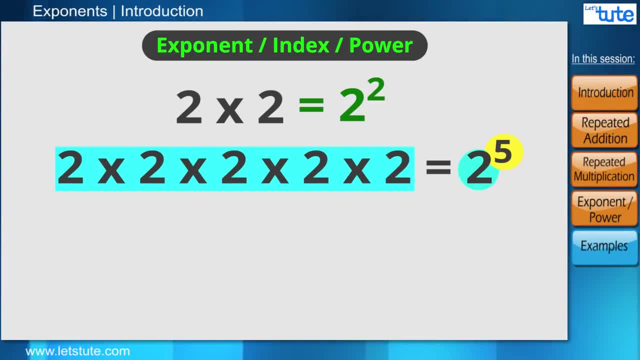 the number 2 has multiplied by itself. or you can say 2 to the power of 5 or 2 to the 5th power. similarly, if it is asked to multiply 2 by 2 for 30 times or 2 by 2 for 50 times, then how you are. 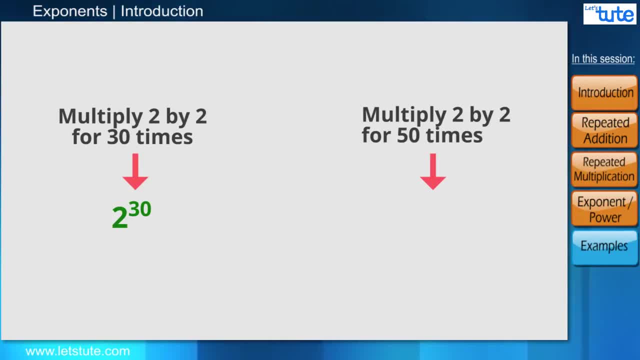 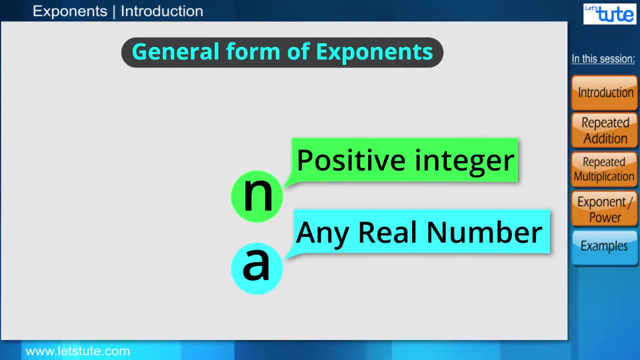 going to write it: 2 raised to the power 30 and 2 raised to the power of 30 and 2 raised to the power 50. right that means for repeated multiplication. we can use exponents in general form. if n is a positive integer and a is any real number, then a raised to the power of n corresponds to repeated. 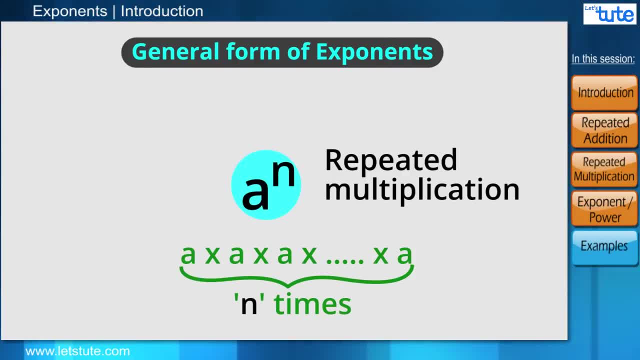 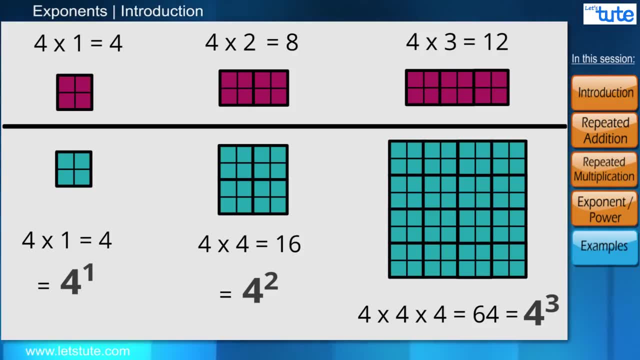 multiplication. friends, there is also one more interesting thing about multiplication and exponential. let's see what is that thing. let's have a look at this image. well, you can see here the number of boxes is increasing rapidly in exponential as compared to multiplication. here, exponentially means if something is increasing or expanding at a sturdy. 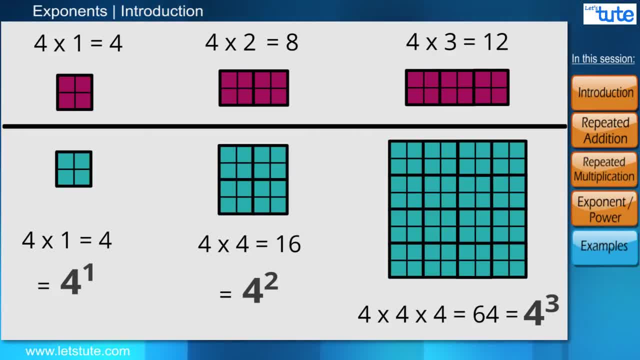 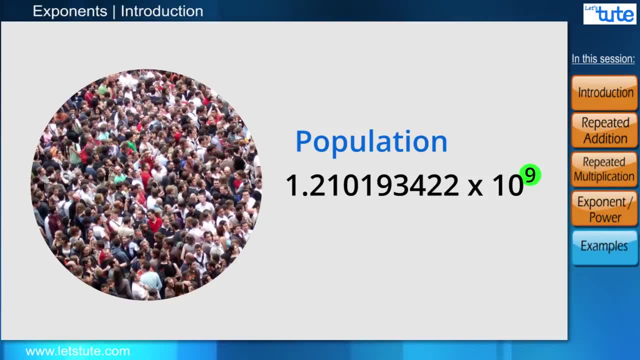 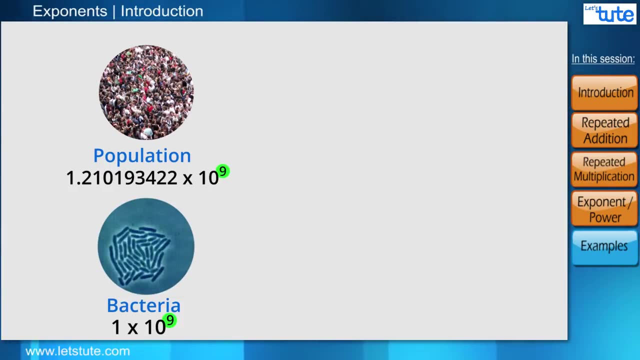 and usually rapid rate, then it is expressed using the exponents. we can even observe in our daily lives, like population grow exponentially each day, or growth of bacteria increases exponentially per hour. similarly, exponents are often used to describe how much memory or RAM a computer holds for.